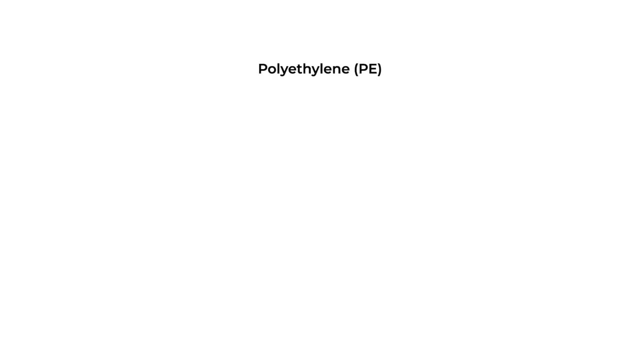 with a real-world example. Let's take polyethylene that we talked about in the intro to this course. The monomer for polyethylene is the hydrocarbon ethylene with a chemical composition of C2H4.. This is reacted together in the proper conditions. 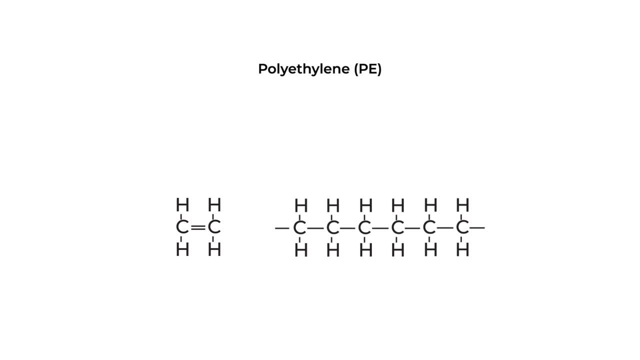 to give us this, our polyethylene chain. Our backbone is our carbon and our side groups are single hydrogen atoms. Therefore, our repeating group looks like this. Sometimes a polymer chain might be written out like this, where our repeat unit is in brackets with subscript N. 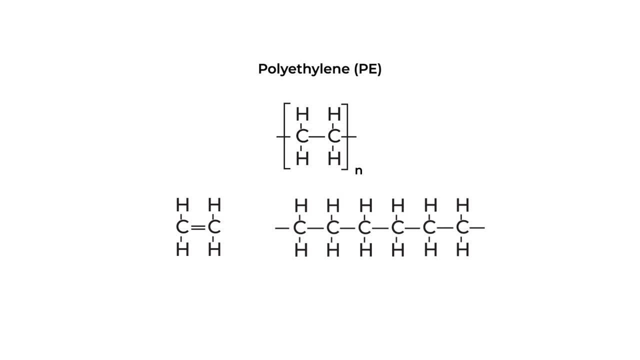 This N indicates the length of our chain. Now, remember that this is a simple drawing that does not take into account our bonding constraints. Our covalent hybridized carbon-carbon bonds are directional, which means we don't have this 180-degree angle. 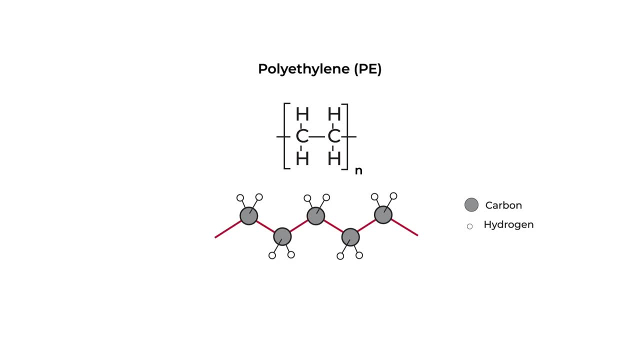 Instead it's closer to 109 degrees like this. Now we said we can change our side groups. We also talked about Teflon in our introduction. We can see the structure and its repeating units. here We've swapped our hydrogens for fluorines. 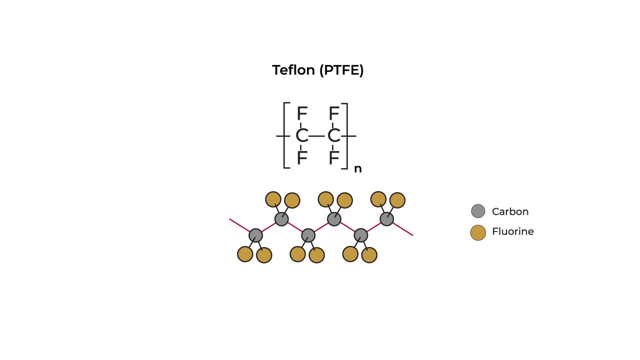 Now for both polyethylene and Teflon. the repeating unit has two carbons, both with the same side groups. Why do we bother showing two carbons? Well, some systems like polyvinyl chloride or PVC have uneven side groups. 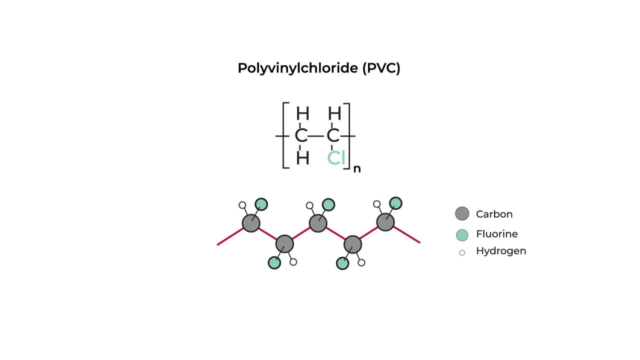 The structure for PVC is shown here. We have three hydrogen side groups and one chlorine side group per repeat unit. Side groups don't have to be just atoms. For example, polypropylene has an ethylene side group along with some hydrogens. 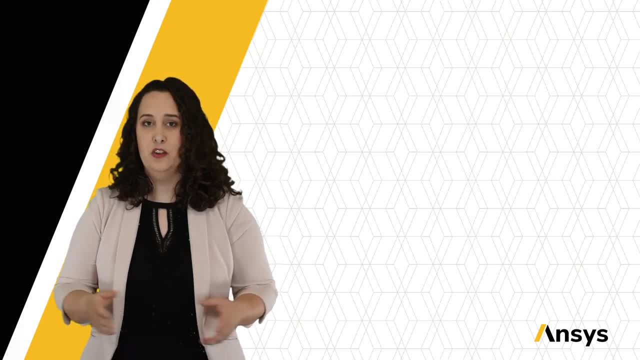 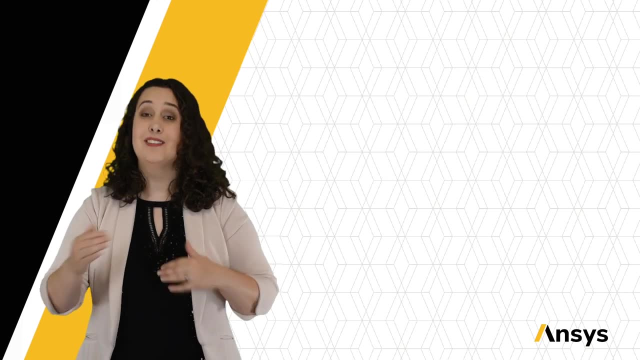 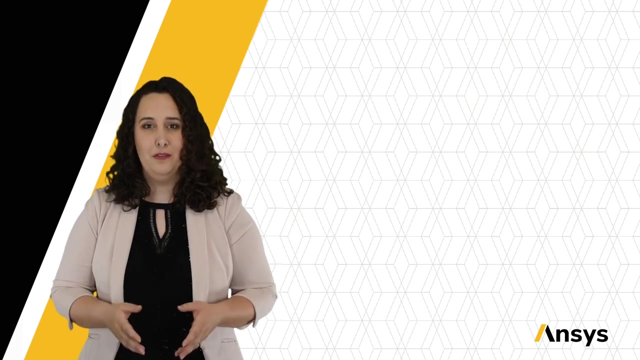 Now these side groups can have multiple configurations depending on how they arrange themselves within the chain, which is called stereoisomerism, or on what side of the chain they arrange themselves on, which is called geometric isomerism. Unfortunately, we don't have time to discuss these today. 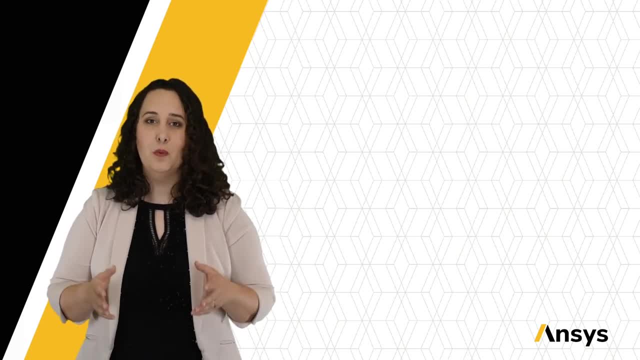 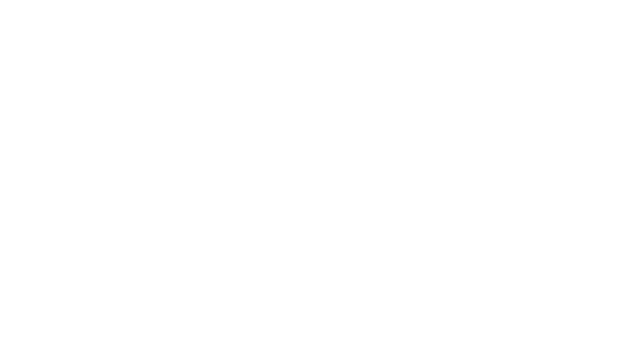 but since we're dealing with three-dimensional bulk materials, we need to be mindful of how these side groups arrange themselves. We also need to be mindful of how our polymers arrange themselves in the bulk material, The linear polymer structure where our chains resemble what's often referred to. 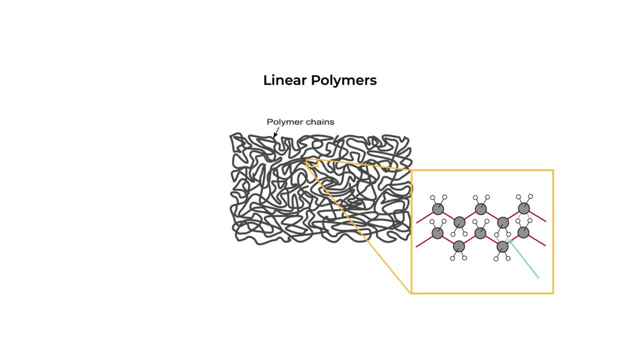 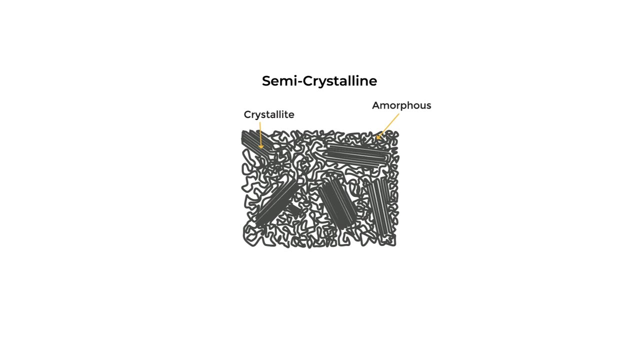 as cooked spaghetti. Here we find our van der Waals, or hydrogen bonds from lesson one between the chains, weakly binding them to one another. When we have linear polymeric chains, we can have a high degree of chain stacking, leading to what's called crystallites. 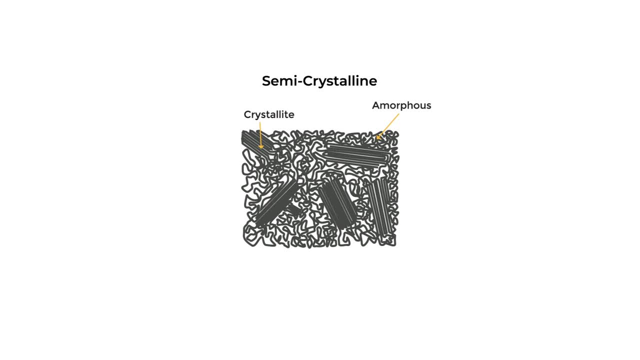 These areas lead to polymers that are semi-crystalline in nature, which alters our polymeric properties. We can also have branched polymers, which again are bonded together by our secondary bonds. The difference is the branched polymers. 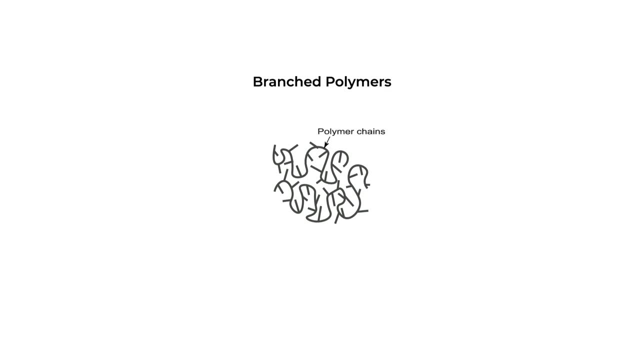 can't pack as closely to one another compared to our linear polymers. Not only does this lead to minimal crystallization, but it also reduces the density of our polymer. For example, our plastic bags from the introduction are made of a low-density polyethylene. 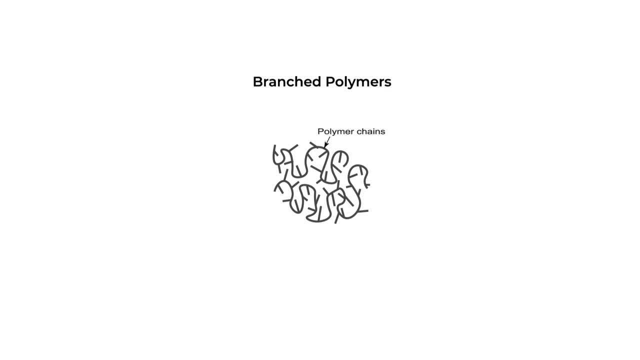 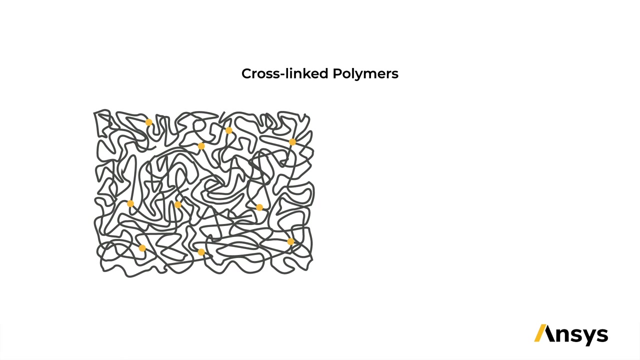 that has this branch structure. High-density polyethylene made with a linear structure is used to reduce wear and friction in total knee replacements Quite a different application for a change in structure. We can also have covalent bonds between our polymer chains. 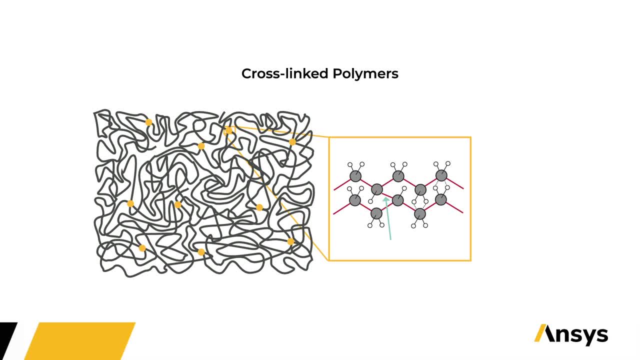 These are called crosslinks. We mentioned our crosslinks at the beginning of this lesson as a difference between thermosets and thermoplastics. Our thermosets don't soften because of these covalent bonds. We need just as much energy to break the covalent bonds. 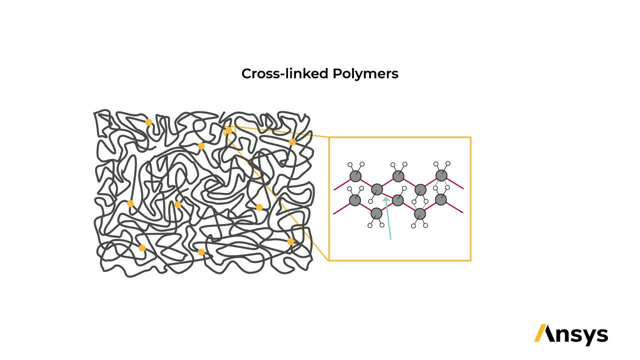 between the chains as we do within the chain, So they all break at roughly the same time. The degree of crosslinking between our chains can vary from low to high. As we get to high degrees of crosslinks we have what's called a network polymer. 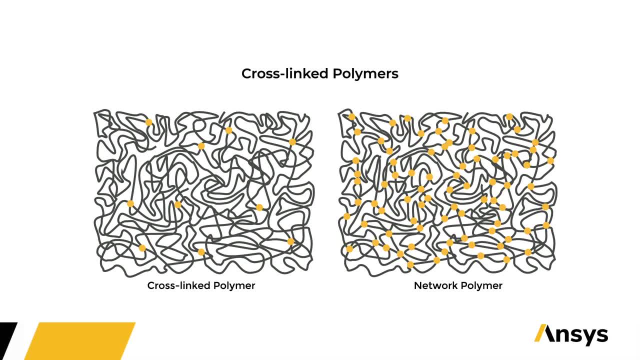 An example of a polymer with a low degree of crosslinking is rubber, which I can stretch and manipulate as an elastomer. A polymer with a high degree of crosslinking is epoxy. I can't stretch epoxy in the same way I can stretch rubber. 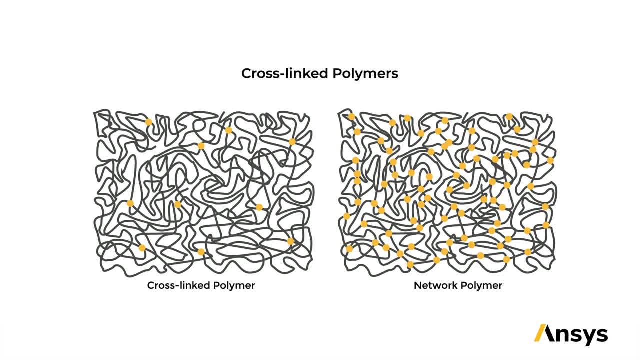 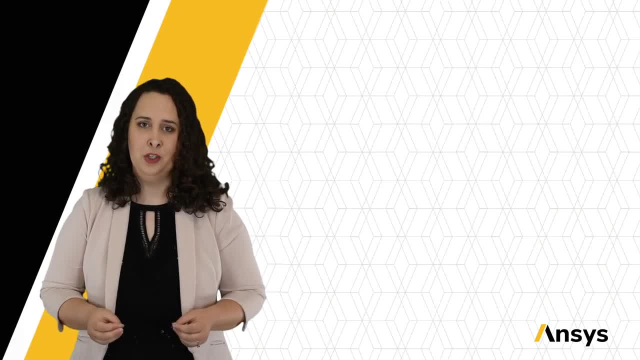 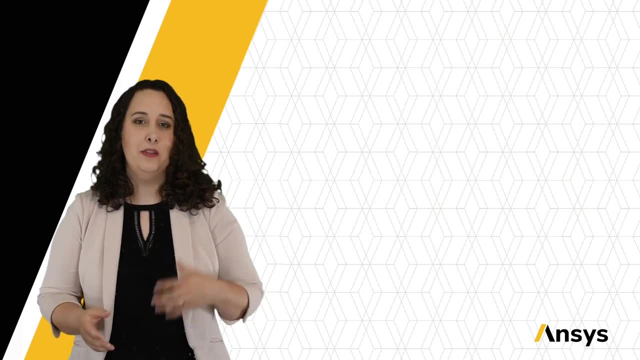 yet they're both crosslinked polymers, So our degree of crosslinking dramatically impacts our performance, And with that we've come to the end of a very terminology-heavy lesson. I know we've talked about a lot of terms, but since polymers can be so varying in their structure,